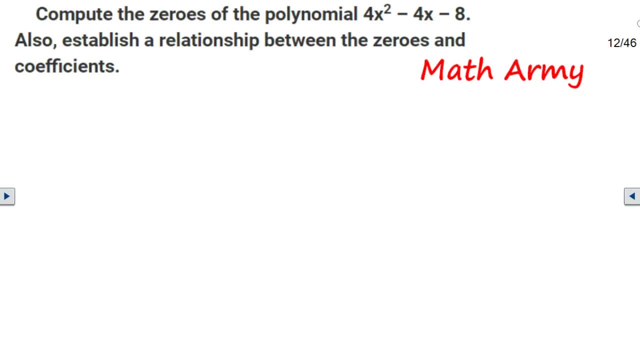 hey guys, welcome to my channel, math army. compute the zeros of the polynomial 4x square minus 4x minus 8. also establish a relationship between the zeros and the coefficient guys. these kind of questions are very regular in our board examination, so let me focus on the given. 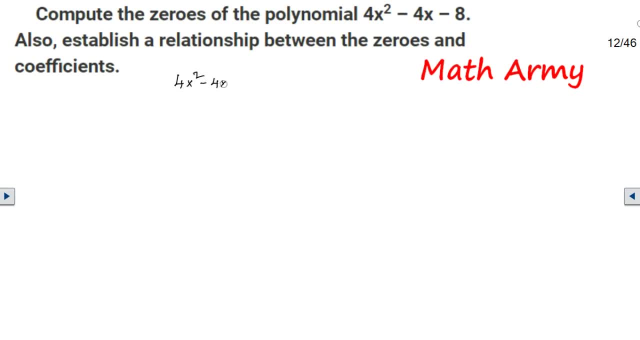 equation first and then. first of all, i'll be focusing on coefficients, and then i will also find the zeros, and later i will try to establish the relationship between these two. okay, now, if you look at the given quadratic equation, a value is 4, b value is minus 4 and c value is 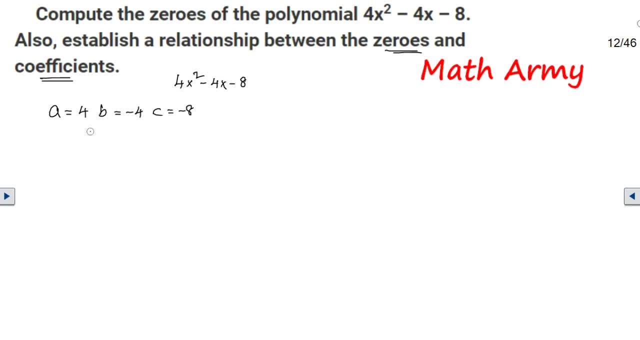 minus 8 right now, as per the formula, the sum of the coefficients. what is the formula? minus b divided by a. so write minus as is, and b value is minus 4. so minus multiplied with minus 4 divided by 4. minus multiplied with minus is plus 4 divided by 4. so the sum of the coefficient is 1. 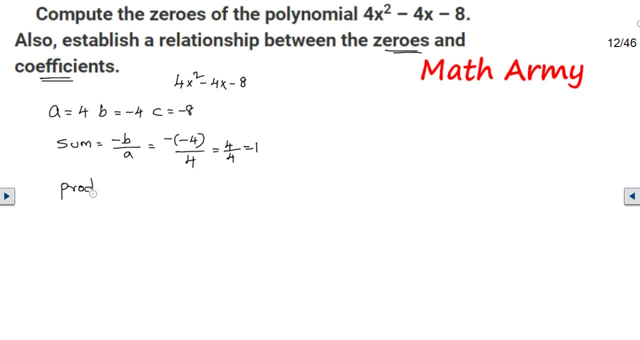 and now the product of the coefficients. what is the formula c by a and c value is minus 8, 4. now 4 divides 8 in 2 times because there is a minus. so the product of the coefficients is minus. now the sum of the coefficient is 1. now let us find the zeros. 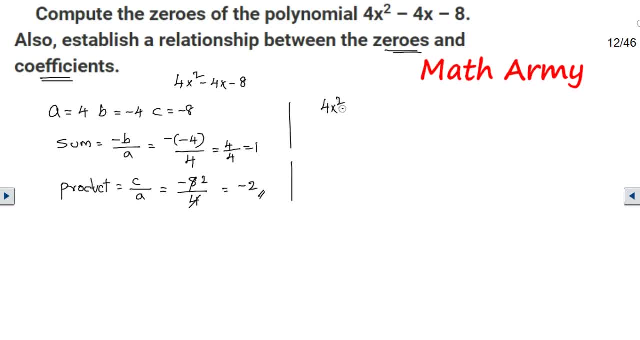 4x square, minus 4x and minus 8. normally you need to equate to the 0 guys. that is a good practice. okay, and now split the middle term, but before that you have to find the zeros and then you have to find the coefficients. so you can see that i can see something common across the given equation. 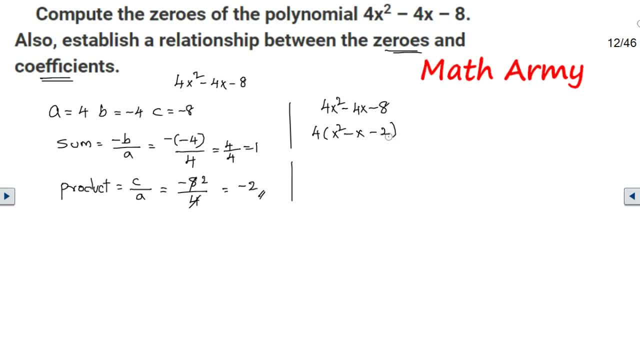 which is 4. so i have taken 4 out. now, if 4 is out, and what is the middle term now? minus x. now split minus x in such a way that the product should be minus 2x square. it's very simple: 2 and 1, if you. 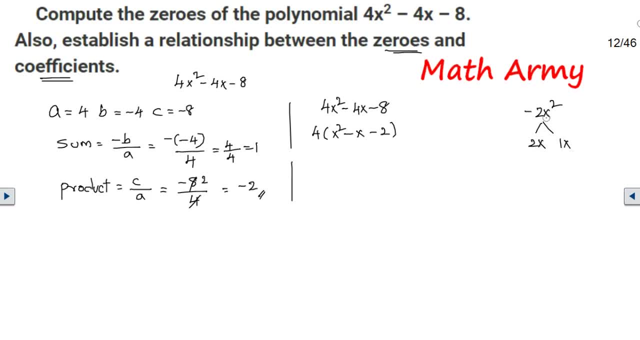 multiply 2 and 1, you are going to get 2.. but you need minus 2.. so put minus before 2 and 1.. the bigger number, which is 2 and plus before 1. now, if you add them, you are going to get minus x. 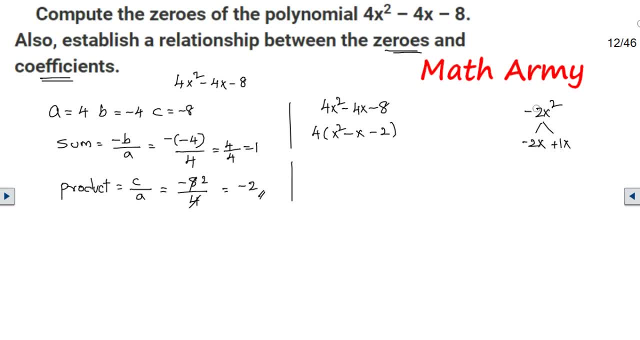 okay, and if you multiply them, you are going to get minus 2x square. and now? so, instead of minus x in the middle term, i am going to write minus 2x plus 1x- okay, and minus 2x minus 2 equal to 0.. 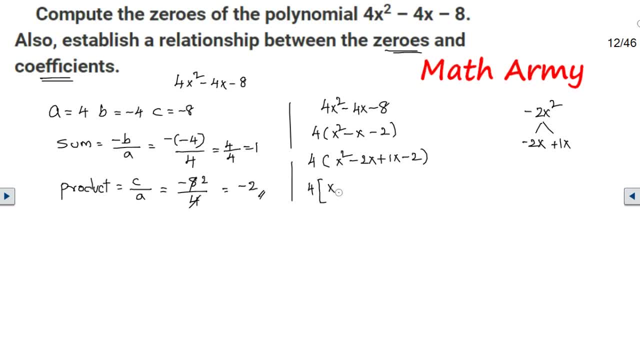 so, therefore, what is our x value? so i am taking x common, so x minus 2 is a factor. and take 1 common, again x minus 2.. now take x minus 2 common, you will be getting the second factor, which is x plus 1.. 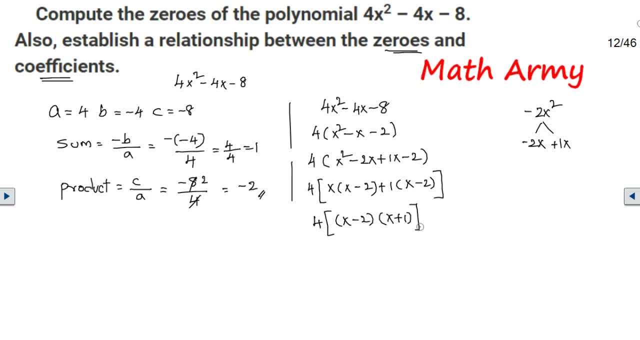 now, as i said in the earlier, you know, equate it to zero. so your x values would be either 2 or x values would be minus 1.. now what you got in the coefficients: the sum sum is 1 and the product is minus 2.. 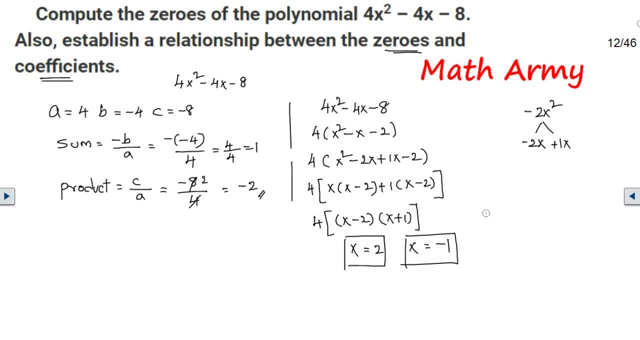 now add the zeros. the sum of the zeros are 2 and minus 1. so add 2 and minus 1, you will be getting 1.. and what is the product of the zeros? 2 multiplied with minus 1, which is minus 2.. now compare the these two values to the sum and coefficient of the. 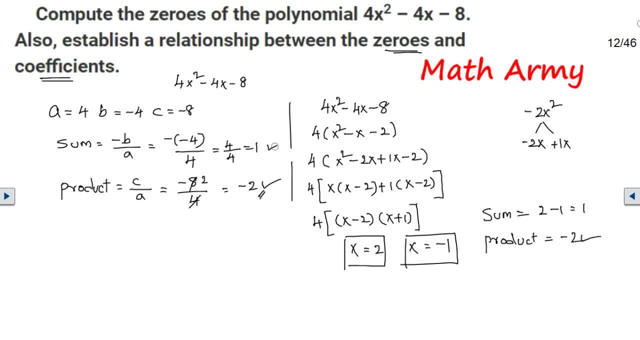 sum and the product of the coefficient. are they matching? yes, and that's it, guys. that is your final answer. i believe you got that, guys. i request you to again practice as many questions as possible, because, though it looks simple, but it is not always so, because if you couldn't able to split, 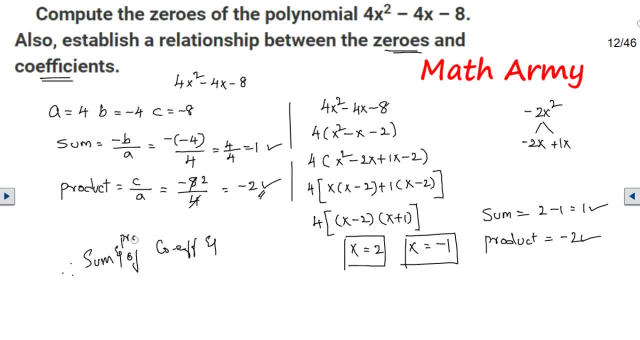 the middle term, then you will be in trouble. you cannot establish the relationship between. so, before leaving, i am writing a statement. sum and product of the coefficients and zeros are matching. okay, and that's it guys. see you in the next video. bye for now, take care you.